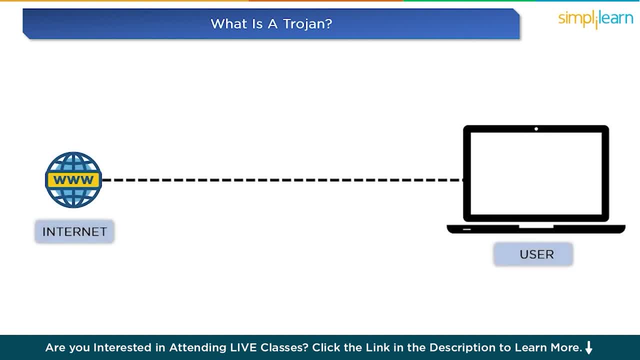 A Trojan is a type of harmful software that pretends to be something useful or desirable while actually being malicious. It's like a sneak imposter hiding inside something you want, like a fun game or a helpful app, Once you unknowingly install it on your computer or 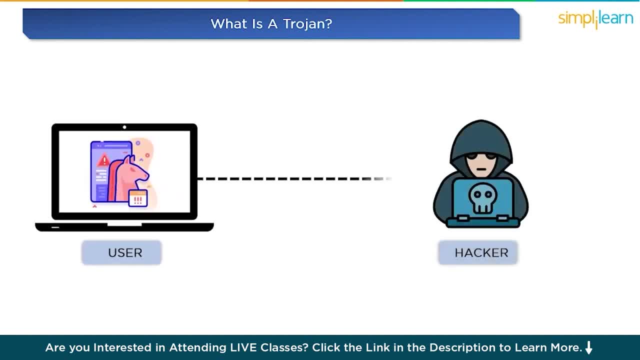 device. it can secretly steal your personal information, Damage your files or give control of your system to hackers without your knowledge. Just like the ancient story of the wooden horse, it looks innocent on the outside but hides dangerous intentions inside. Now that we know the basics, let's look at the 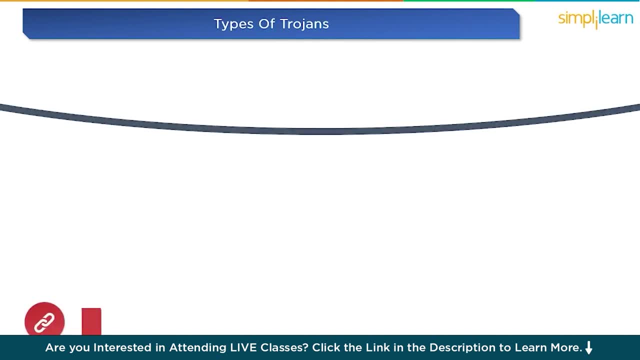 different types of Trojans out there. The first one is remote access Trojans, or rats. These sneaky Trojans allow hackers to gain unauthorized access to a victim's computer remotely. They can spy on users, steal sensitive data and even control the infected. 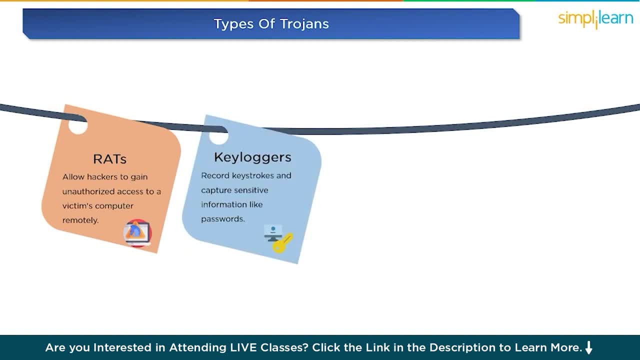 system. Keylogger's Trojan silently records keystrokes, capturing sensitive information. It's like password, credit card numbers and other personal data. They can be incredibly dangerous, especially if you use online banking or make online purchases. Backdoor Trojans- Backdoor. 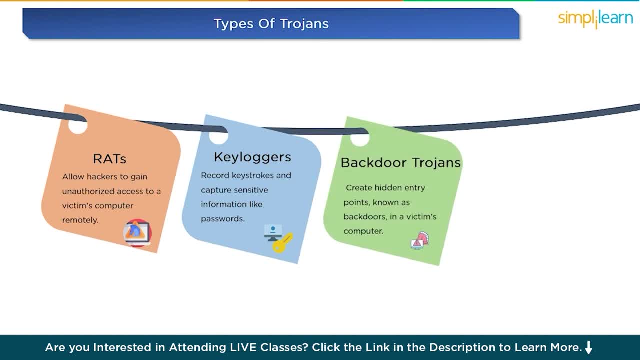 Trojans create hidden entry points, known as backdoors, in a victim's computer. Once installed, they grant cybercriminals full control over the infected system, essentially leaving it wide open for further attacks. The last one The Trojan is Downloaders: Downloaders, as the name suggests, download additional malicious. 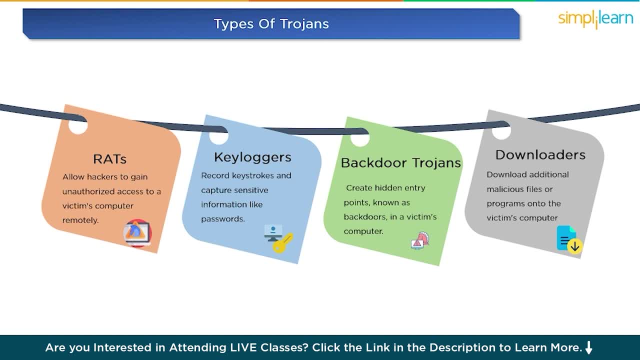 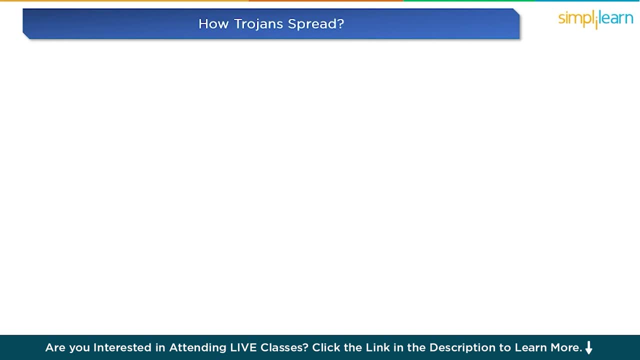 files or programs onto the victim's computer. They are often used to deliver more harmful malware to the system, So you might be wondering how the Trojan spreads in the first place. So let's shed some light on that. The first is phishing emails. Phishing emails are one. 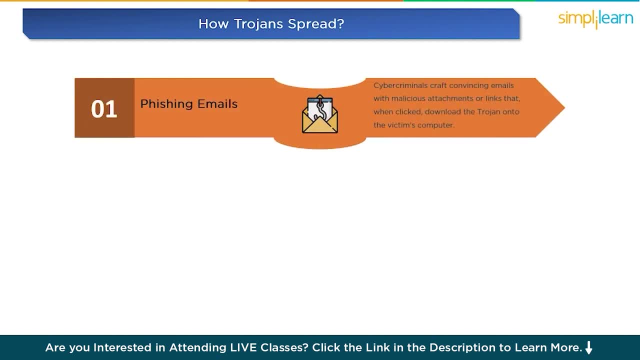 of the most common ways Trojans infiltrate systems. Cybercriminals craft convincing emails with malicious attachments or links that, when clicked, download the Trojan onto the victim's computer- Malicious websites. Visiting compromised or malicious websites can also lead to unintentional 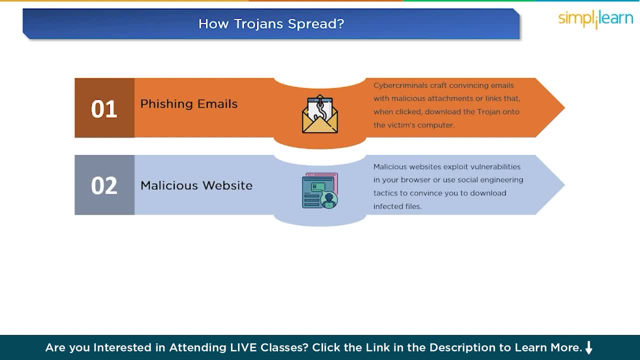 Trojan downloads. These sites exploit vulnerabilities in your browser or use social engineering techniques to convince you to download infected files. The third one is software downloads. Even seemingly legitimate software downloads from untrustworthy sources can be infected with Trojans. Always download software from official and reputable websites. Also, if you 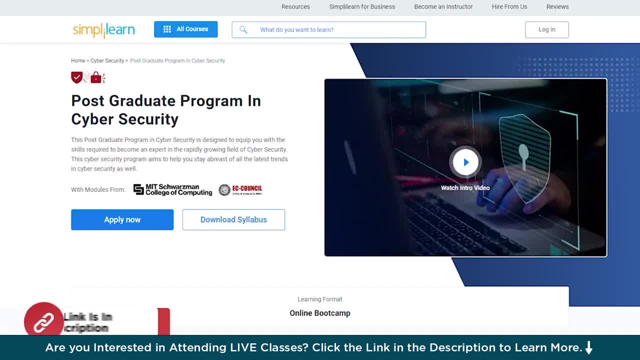 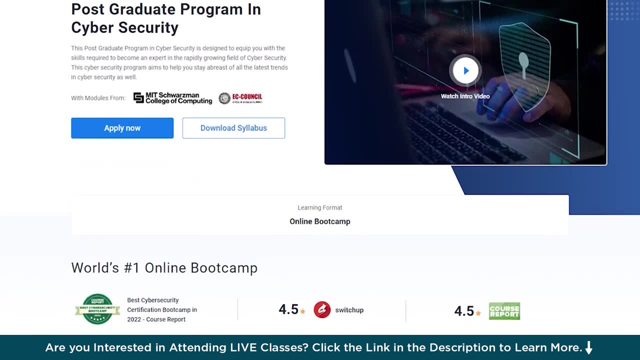 want to master the field of cybersecurity, then simply learn how to download software from a software library. Simply Learn's postgraduate program in cybersecurity in collaboration with MIT is clearly the right choice for you. This postgraduate program in cybersecurity is designed to equip you. 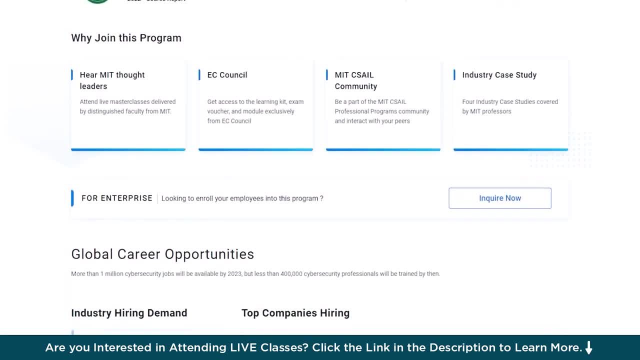 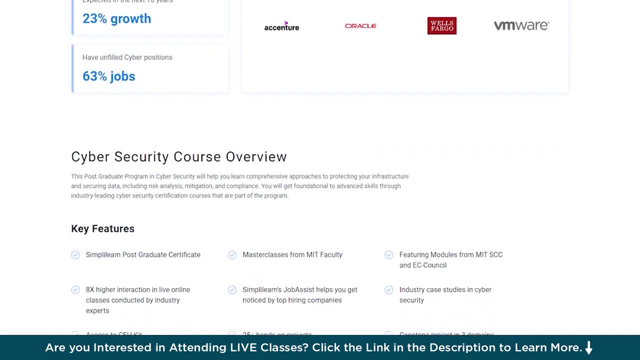 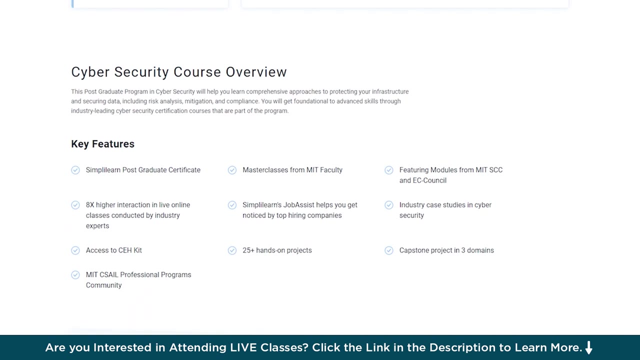 with the skills required to become an expert in the rapidly growing field of cybersecurity. This cybersecurity program aims to help you stay ahead of the latest cyber security threats. Key features of this program are Simply Learn's postgraduate certificate master classes from MIT faculty featuring modules from MIT, SCC and EC counsel. 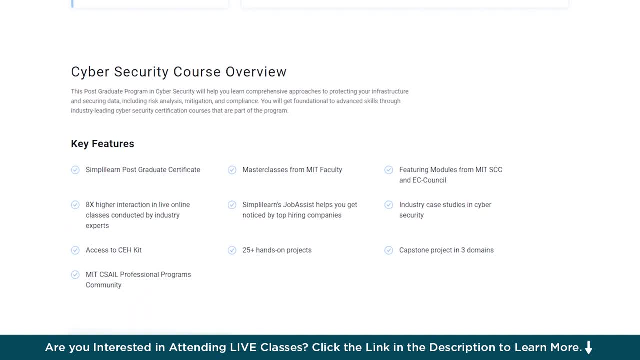 Simply Learn's postgraduate certificate also includes a Google training course. This programme will be available as one of the first courses in the CSE program, as well as thestreams for access to ch kit plus 25 hands-on projects. the cyber security certification program begins with. 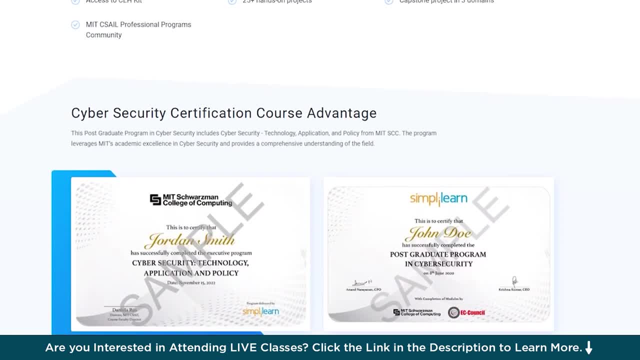 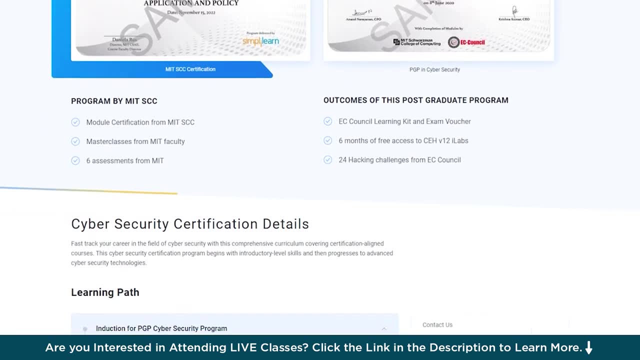 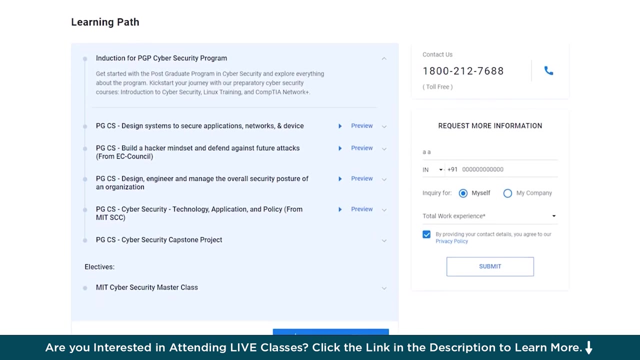 introductory level skills and then progresses to advance cyber security technologies. this program covers all the essential skills you will need to become an expert in the field of cyber security. cyber security is definitely one of the top concerns of businesses today, in any industry- from securing data to anticipating cyber attacks and placing enterprise-wide safeguards to prevent. 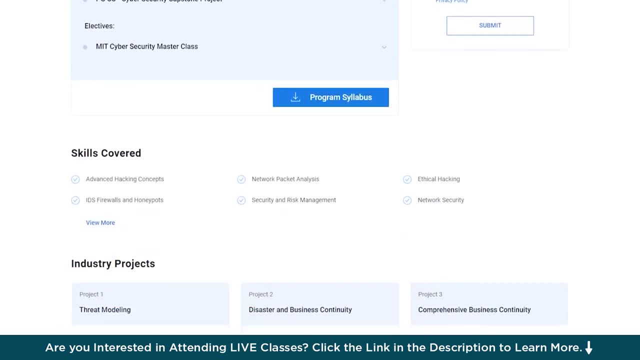 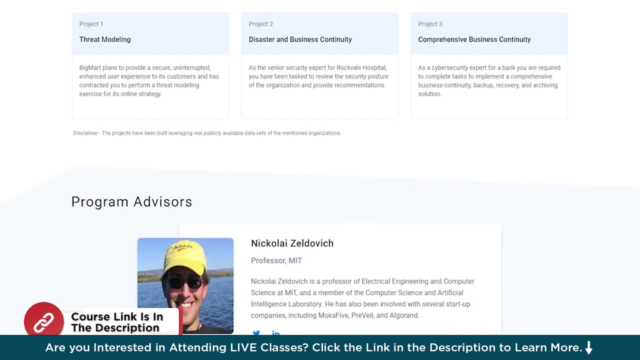 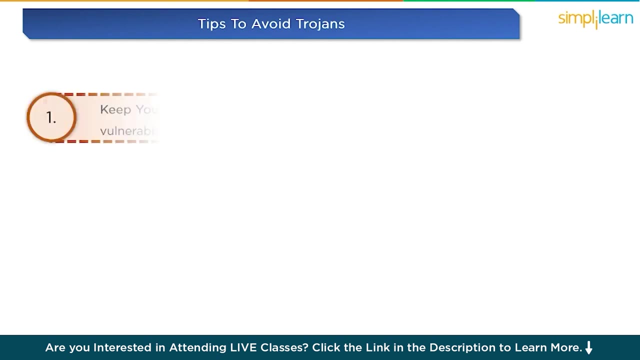 them. employers worldwide are increasingly looking for qualified cyber security professionals to join them. so what are you waiting for? find the course in the link mentioned in the description box below and enroll today. now that we understand the potential risks, let's explore some essential tips to protect ourselves from trojans. number one is keep your software updated regularly. update. 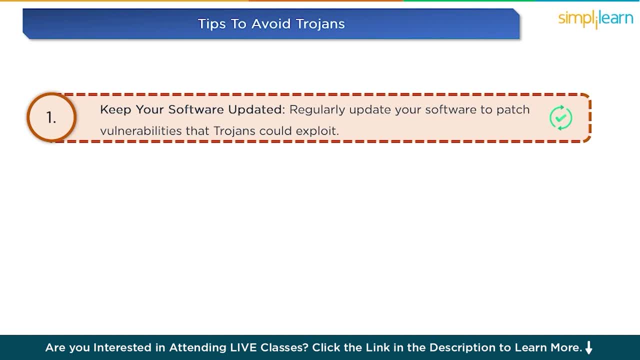 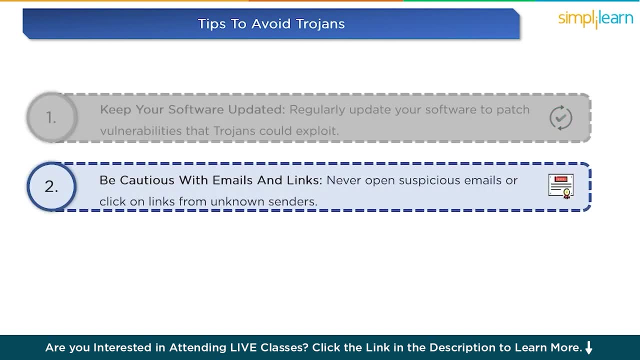 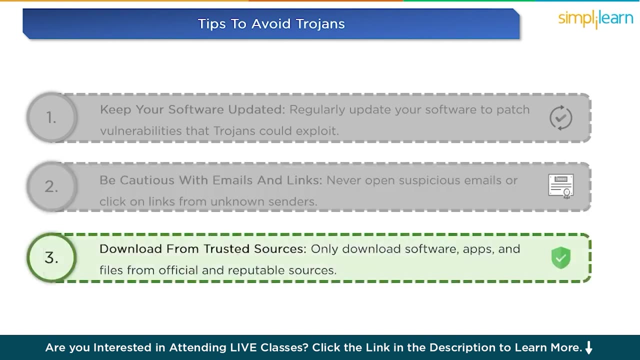 your operating system, web browsers and security software to patch vulnerabilities that trojans can exploit. be cautious with emails and links. you never open suspicious emails or click on links from unknown senders. verify the center's identity before opening any attachment. third is download from trusted sources. only download software apps. 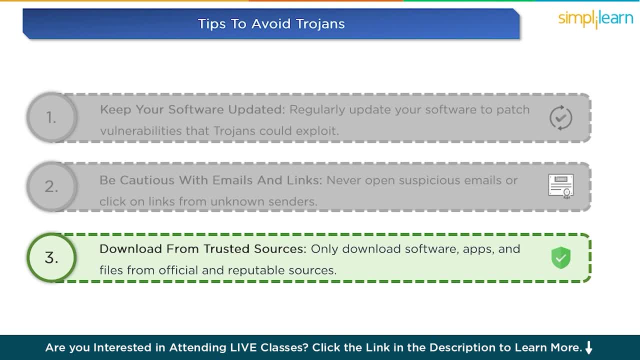 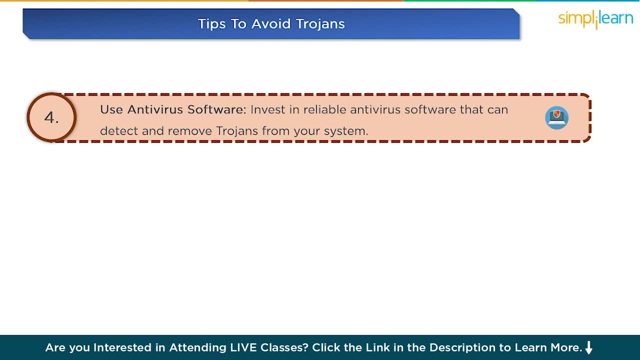 and files from official and reputable sources. avoid shady websites and torrents. fourth is: use antivirus software. invest in reliable antivirus software that can detect and remove trojans from your system. in conclusion, trojans are dangerous and deceitful cyber threats that can cause severe damage to your computer and compromise your personal information. however, 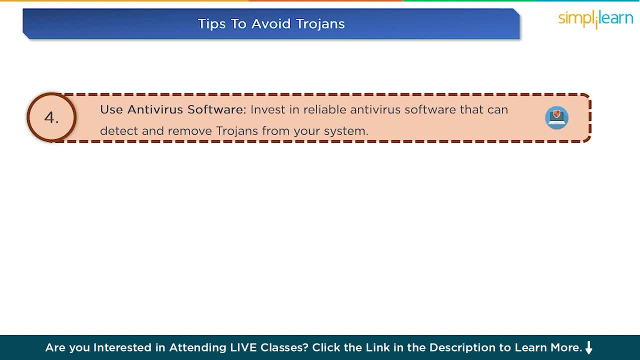 armed with knowledge and proper security measures, you can protect yourself from falling victim to these malicious attacks. a lot of individuals have attained high salaries and better career opportunities through our postgraduate program in cyber security in collaboration with mit university. so let's hear from one of those graduates. hi, i'm philip, i'm 61 years old and last year i upskilled. 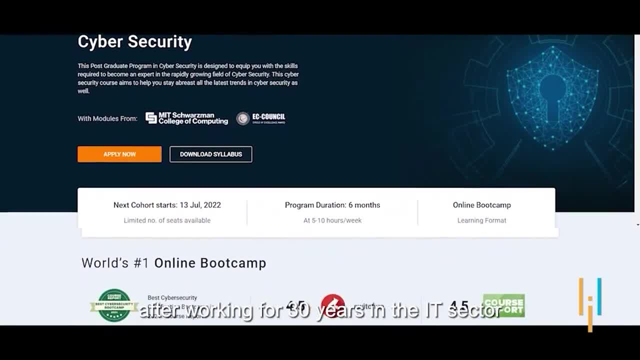 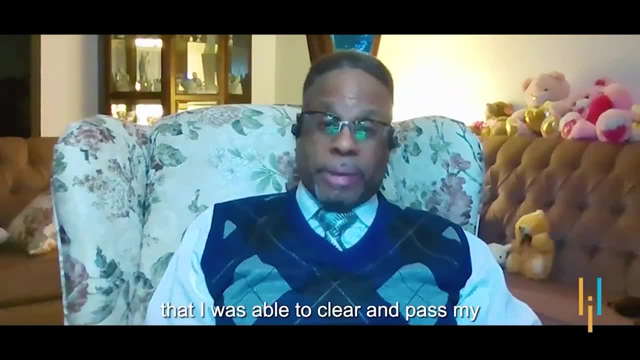 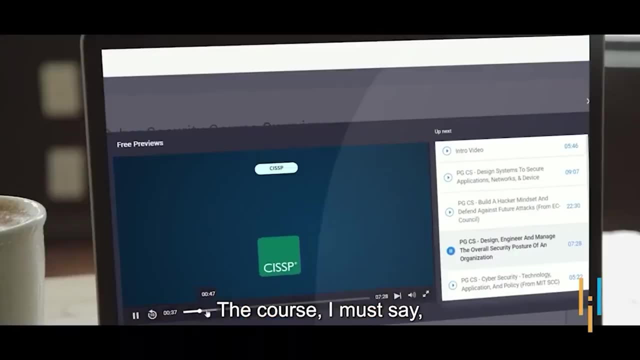 project. i was going to simply learned postgraduate program in cyber security after working 30 years in the it sector in various different profiles. i'm happy to tell you that i was able to clear and pass my cisp and ccsp certification exams on the first attempt after taking the course. course i 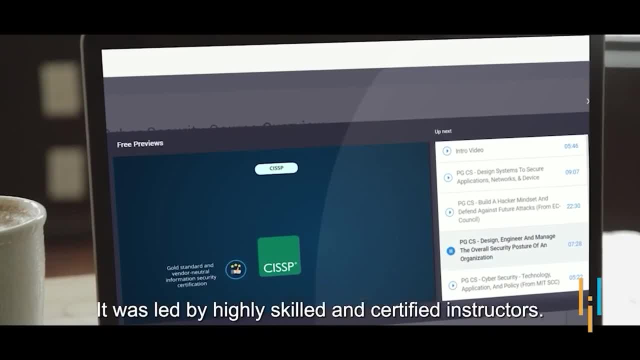 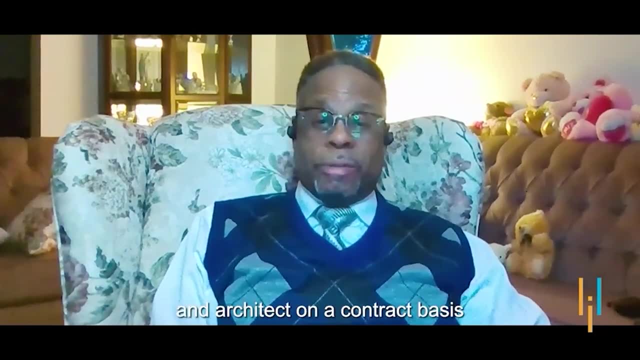 must say, was packed with practical examples. it was led by highly skilled certified instructors. i worked with many companies before- security analysts and the architect- on a contract basis, but i needed some stability. i would say to be able to pass my cisp and ccsp certifications on a contract basis, but i needed some stability, which i could do. 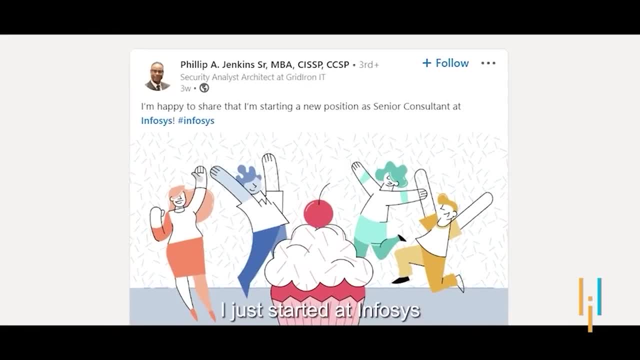 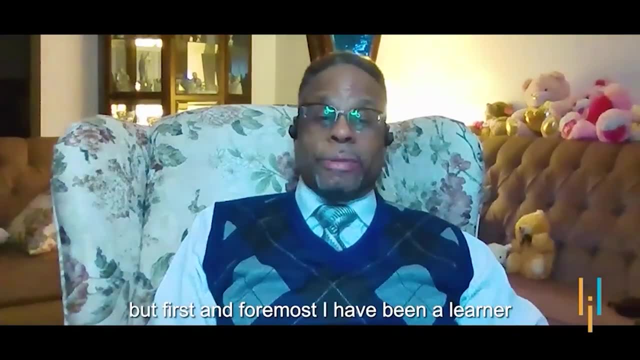 I needed some stability, which I got with the job I just started with Infosys as a cybersecurity consultant Happened after I took the course. But first and foremost, I've been a learner. Be a learner first. And that's all for this video. Remember: always stay vigilant and take 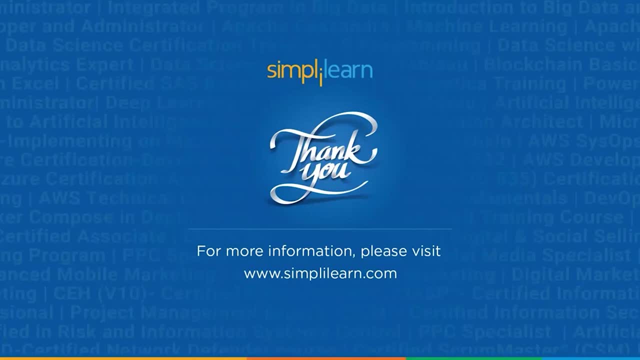 precautions when using the internet to ensure your online safety. Thank you for joining us today as we delved into the world of Trojans. If you find this video informative, don't forget to give it a thumbs up and subscribe to our channel for more exciting content. We'll see you next time, Until. 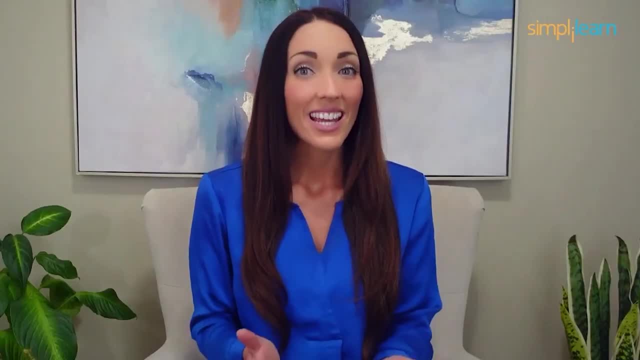 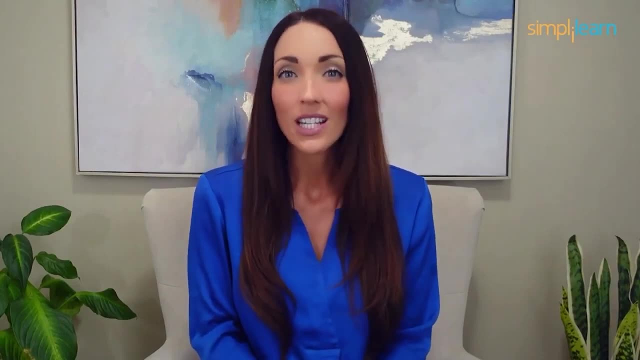 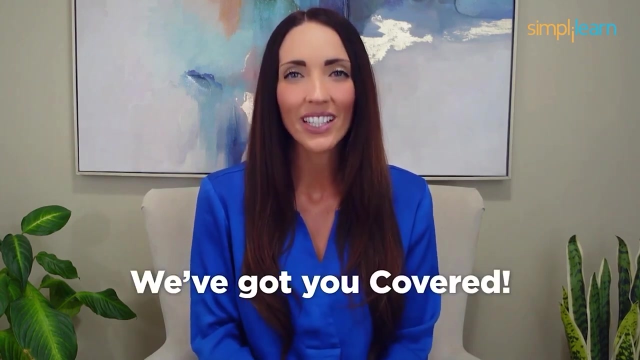 then keep learning and stay tuned to Simply Learn. Staying ahead in your career requires continuous learning and upskilling. Whether you're a student aiming to learn today's top skills or a working professional looking to advance your career, we've got you covered. Explore our.